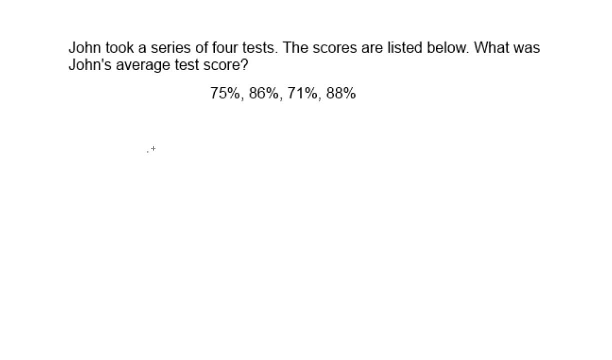 Alright. so we're going to be talking about averages. Obviously, to take an average, we're going to add up all the numbers and divide by however many numbers there are. So this first one. it says John took a series of four tests. The scores are listed below. What was John's average test score? So I see here that he's got 75,, 86,, 71, and an 88. If I add these numbers together- 86 plus 71 plus 88, I'm going to get an average of 75.. 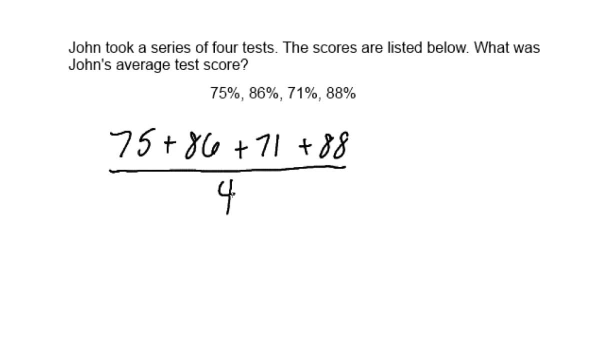 And then I'm going to divide these numbers by four, because there are four tests. I'm going to set this equal to X. And the reason I'm setting it equal to X is because this is what I'm actually looking for. I don't actually know the average, So that is my variable. So I'm adding up these four top numbers And if you add 75,, 86,, 71, and 88,, you'll end up with 320.. And this is still being divided by four. I'm just dropping it down. It's still equal to X. 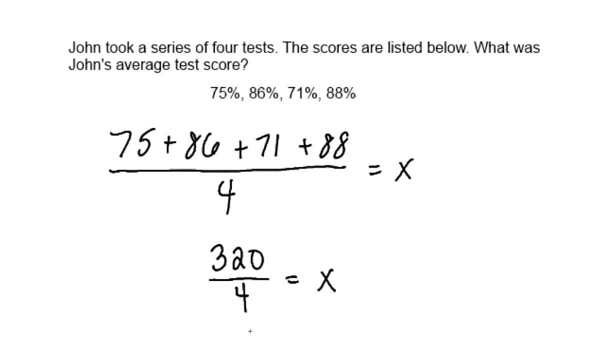 And if you take 320, divide by four, you end up with 80.. So 80 would be the average test score. But let's say I'm not given a test score, Let's say that I'm given the average. So notice that we are looking for the average here. We're missing the average. But let's say I get an example where they give me this number but I'm missing one of the test scores. So something like this: 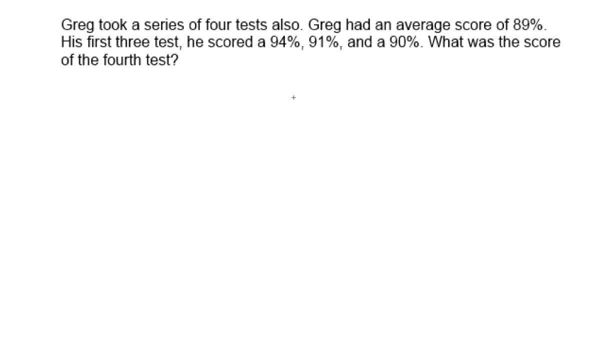 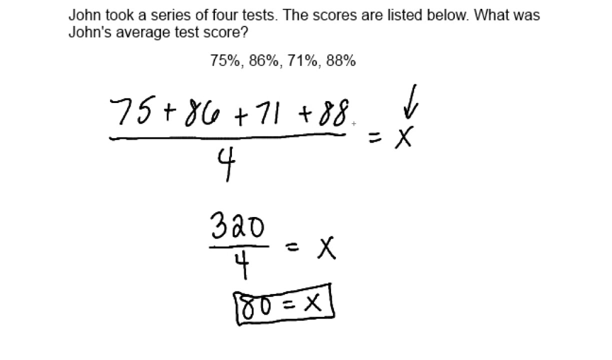 It says Greg took a series of four tests. also, Greg had an average score of 89. So there's my average. His first three tests he scored a 94,, a 91, and a 90. What was the score of the fourth test? I'm going to set this up exactly like I did in the first example. If you notice, I had the four tests listed up top divided by the four, which was the number of how many tests there were, And I set it equal to X. 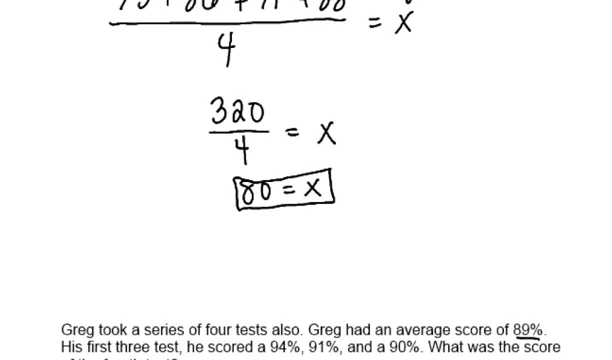 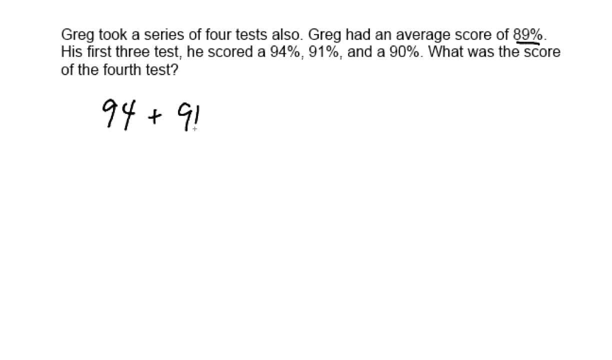 The average, which I didn't know in this case. Well, in this one, I'm going to set it up the same way. I'm going to say I've got a 94 plus a 91 plus a 90. And I don't know this fourth test score, So I'm going to make that my variable. That's what I'm looking for, And it's still being divided by how many tests there are, which there are four, I just don't know this one, And I'm going to set this equal to, we know, the average. 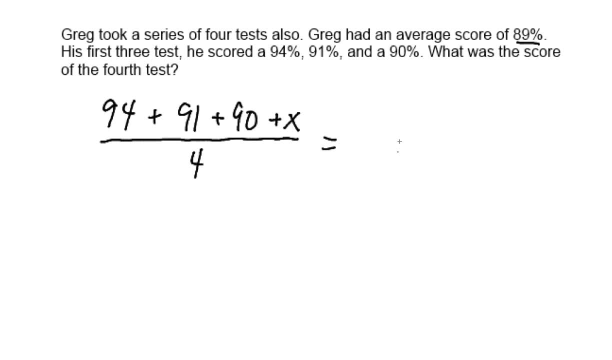 In the last example. I put the average right here And it was X, because that's what I was looking for. But now it's going to be the 89. And now I'm just going to simplify this as much as I can down and try to isolate the X. So I'm going to first start off by adding these three numbers up top: the 94,, the 91, and the 90. If I add those three numbers together I get 275.. I still got this plus X. I'm going to write plus X on the end. This doesn't matter. 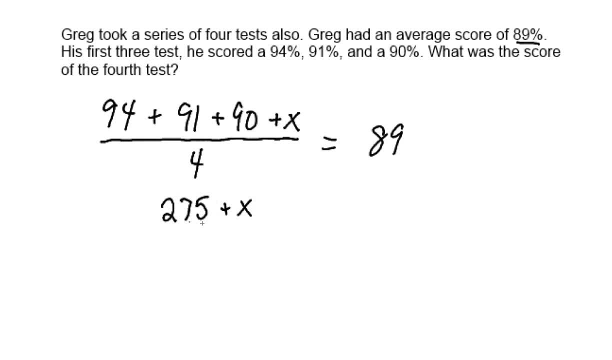 This doesn't combine variables and constant terms like 275 do not combine And it's still being divided by four And I still have the 89 on the right side. My next step: I want to get rid of this four, So I need to multiply because this is being divided. The four is being divided from the 275 plus the X, And I undo division with multiplication, So I'm going to take this entire thing and multiply by four. 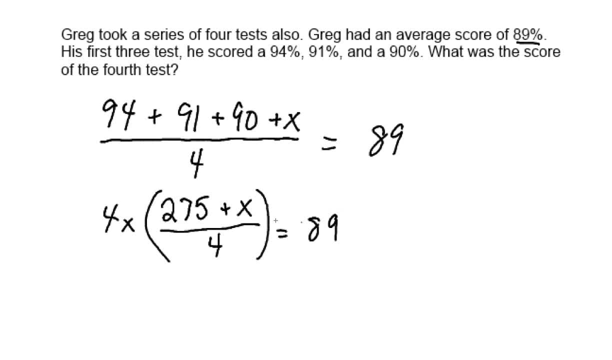 Which what I do to one side, I have to do to the other. So if I've multiplied this entire left side by four, I also have to multiply the entire right side by four. And on this left side, it's a pretty easy occurrence here where the fours are going to cancel each other out. You've got the numerator, This four is being multiplied to the numerator, But there's a four on the denominator, So they end up canceling, which will leave you with 275 plus X.